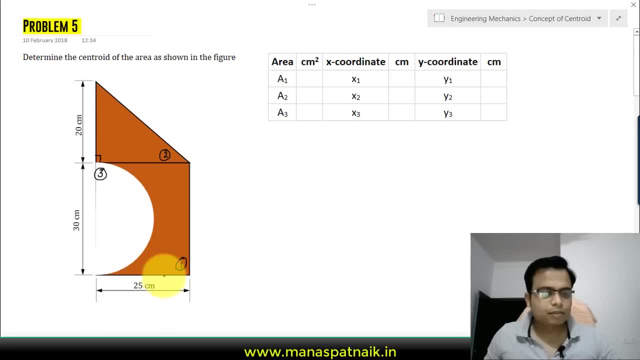 This is the rectangle I'm talking about. The base of the rectangle is 25.. The height of the rectangle is 30. So 25 multiplied by 30 is obviously going to be 750.. Well, the unit is centimeters square. Secondly, when you speak about this area of this triangle, area of the 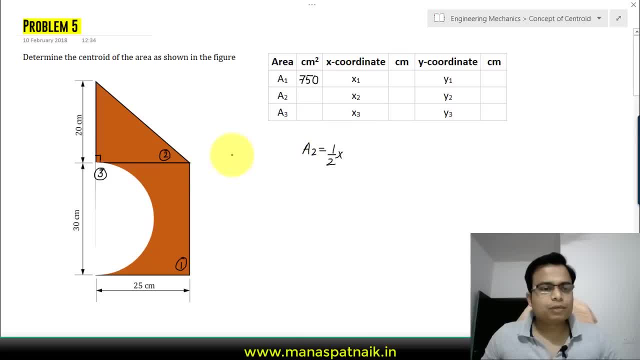 triangle, let's say, is a two, is equal to half of base basis. How much from this point to this point? This is the base and which is equal to how much? 25.. That's 25 multiplied by the height. This height, from here till we reach here, is 20.. 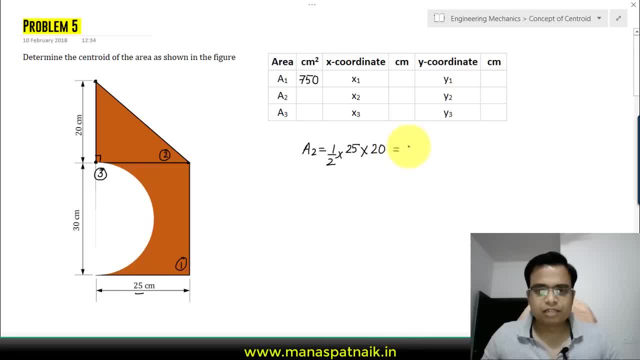 So that's pretty simple, That's 500.. 500 over 2 is 250.. So area 2, let's say, is 250.. And then, finally, we have area 3.. Well, A3 is equal to its area of a semicircle, So it's going to be pi? r. 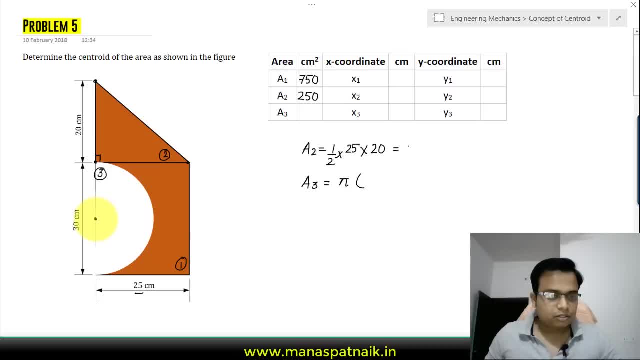 square. How much is the value of r? You see, this is the center. This is precisely the radius. Now, if the diameter of the semicircle is 30, then the radius has got to be 15.. So pi r square divided by 2. Put this up into a calculator And the 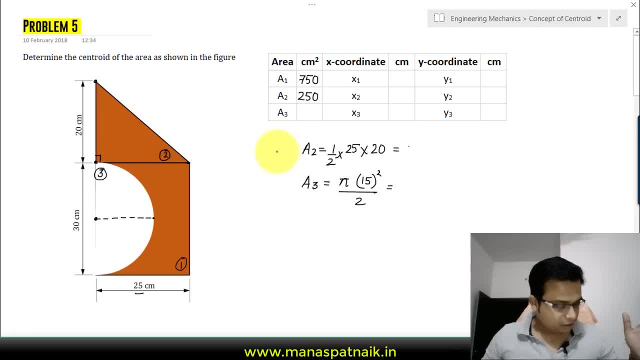 final value of area that you're going to get is: let me check how much it is: It's 353.43.. Let me write this: 353.43.. Okay, now let's proceed and let's get the values of x and y coordinates. For that, what needs to be done is: 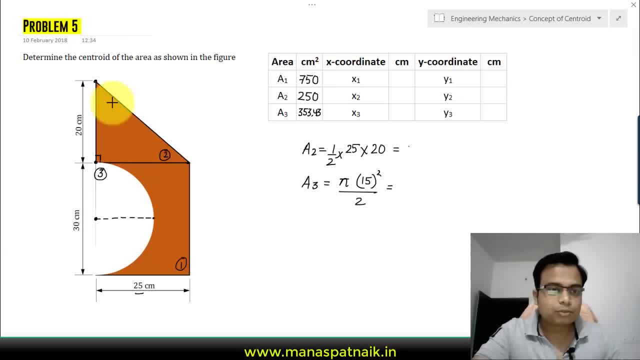 let me have a coordinate axis initially. Okay, this looks pretty good. Yeah, something, something of this sort, And let me bring this closer And this will do the job. Yeah, that's it, And let me write over here. This is y. 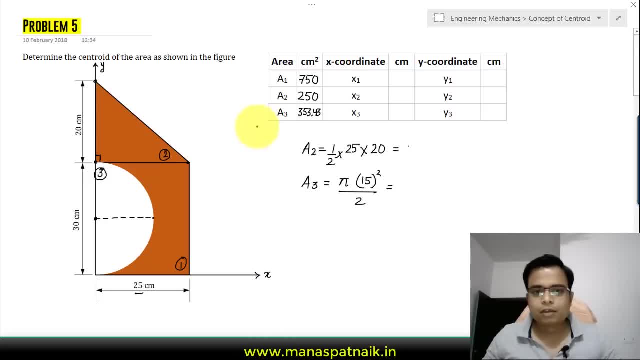 And this is x. So what do we need to work out? We need to work out x1.. If you look at this rectangle over here, the 25 by 30 rectangle, it will have its centroid somewhere here, Okay, somewhere here. Now, this for the rectangle is x1.. And this for the rectangle is y1.. 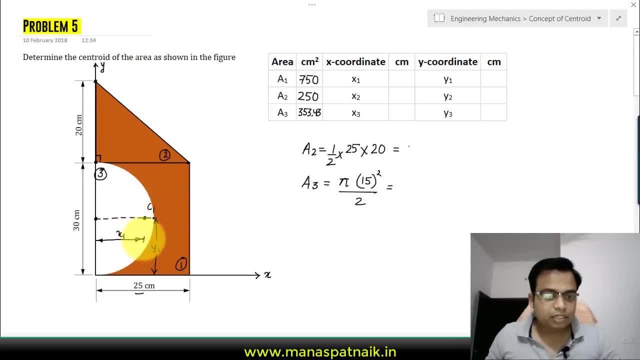 If I say that this is centroid 1 for the rectangle, how much is x1?? Half of 25.. So half of 25 is 12.5.. That was pretty simple. And what about y1? y1 is going to be half of the height of rectangle. So 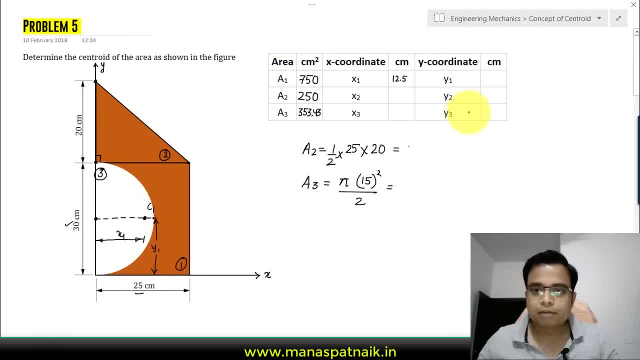 the height of rectangle is 30. So half of 30 is obviously this is 15.. Now let me check this: 12.5 and 15.. Yeah, Good, Now let's go ahead and let's try to work out centroid of this triangle. 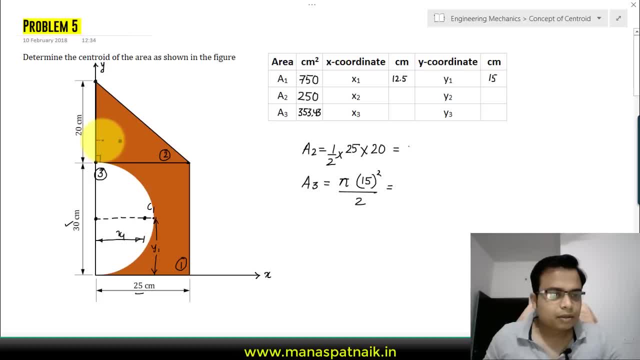 Now, the triangle centroid will be somewhere here. Okay, This distance and this distance. Okay, Now let me tell you something about the triangles, or, to be very precise, the right angle triangles and their centroids. The centroids are always measured from the right angle. Okay, let's say this is B. 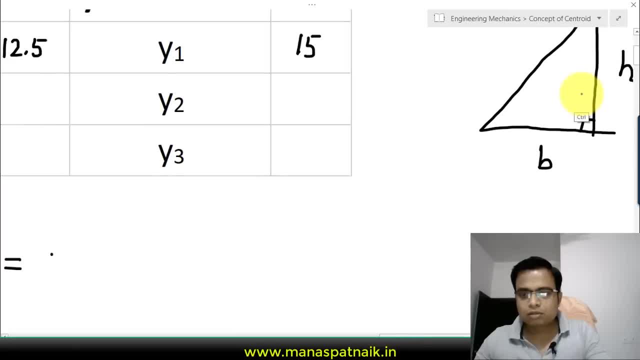 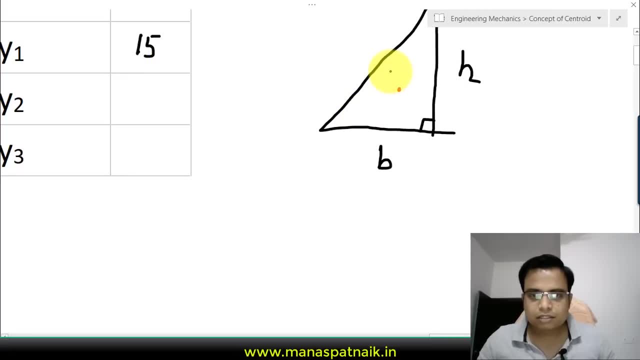 And let's say this is H- Let me zoom on this- And it's a centroid will be somewhere here you can use a different color. Okay, say this is the centroid and this is going to be the x coordinate of the centroid and this is going. 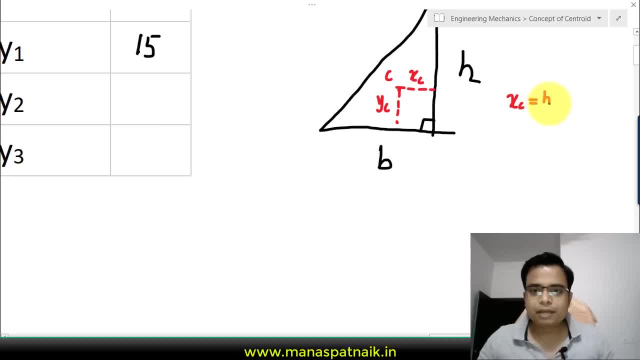 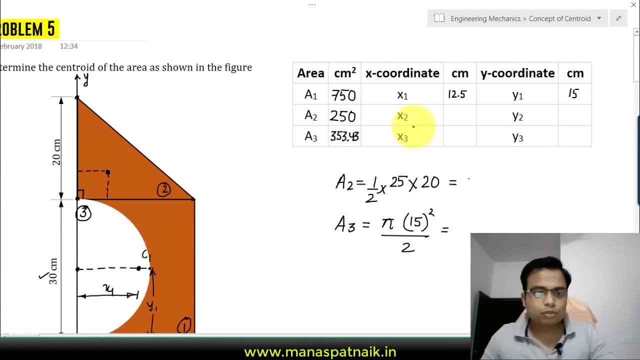 to be the y coordinate. x c is equal to h by 3, not h by 3, but p by 3, whereas y c is going to be h over 3. that's it always measure the centroid from the corner, which has the right angle. okay, this is the best way to approach now in the same manner. 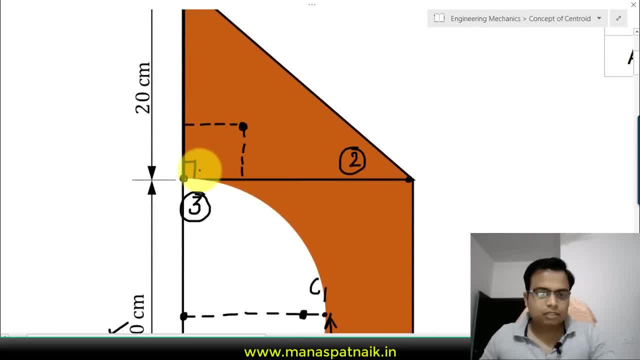 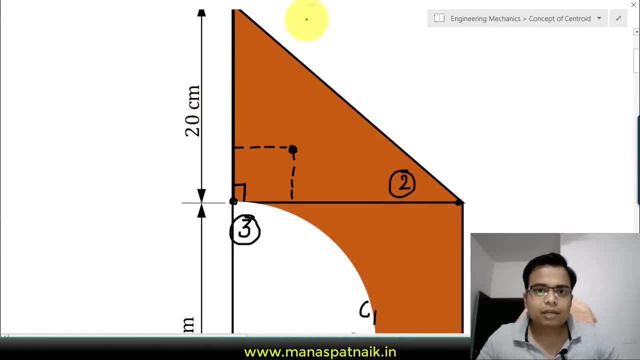 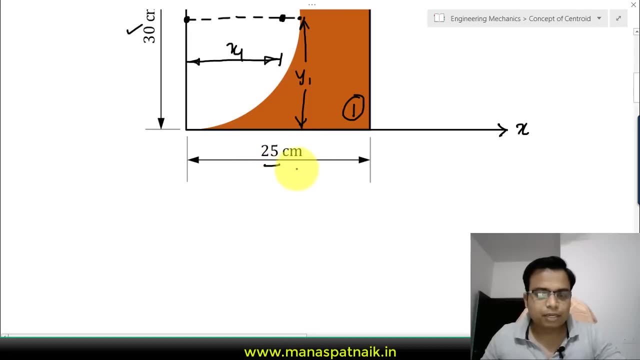 this distance. this distance is going to be. this color is not matching. let me use a different color. let me use a black color. this is going to be. let me see, that's 25. okay, so the base of this triangle is 25. from here till we reach here, that's 25. so this has got to be 25 divided by 3. 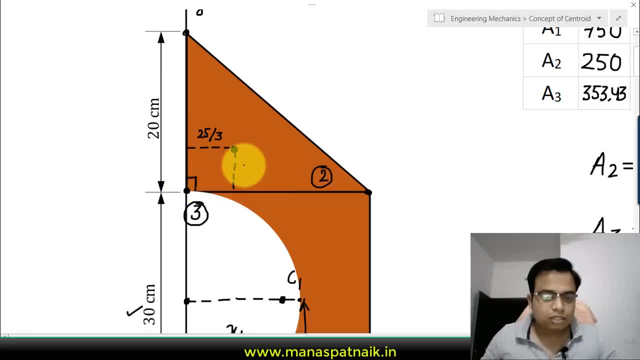 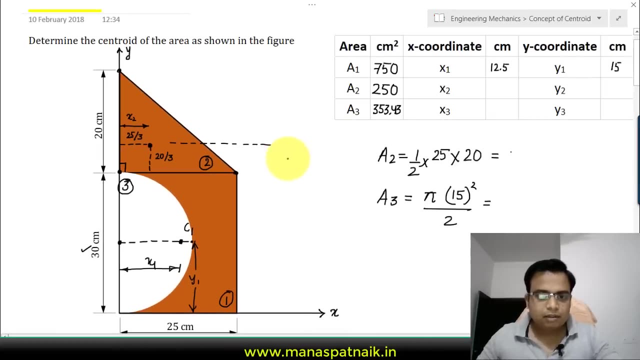 and this distance, that is the height. height is how much? 20. so this has got to be 20 over three. now this automatically qualifies for x2 and as far as this y2 is concerned, y2 can be calculated, but for that I need to draw a line. let's see if I can make a. 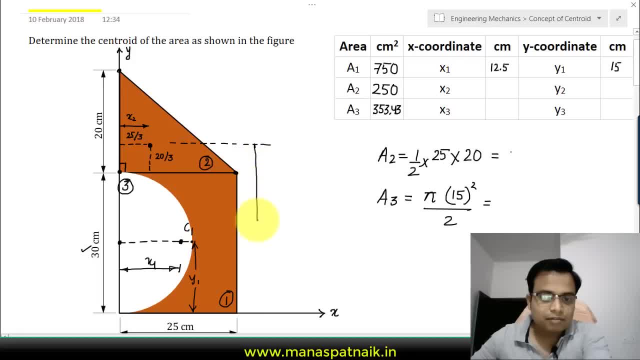 straight line. well, that is y2. that is y2. okay, so if I were to calculate the value of y2, it would be something like this: y2 will be equal to: from here till we reach here. that is how much. that's 30, and plus this distance from here till we reach here, which is how. 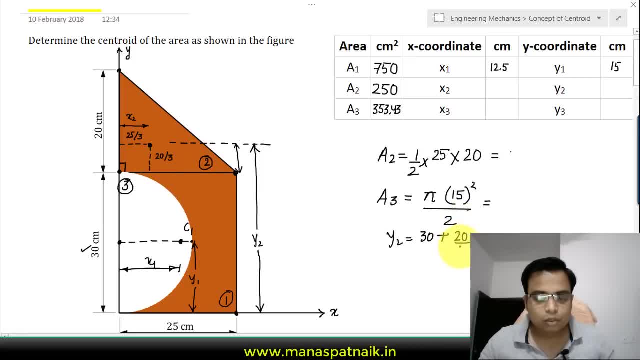 much 20 over 3, so 30 plus 20 over 3. okay, put this up into a calculator and the final value that you will get of y2 is 36.67. that is 36.67. let me write it over here: 36.67. 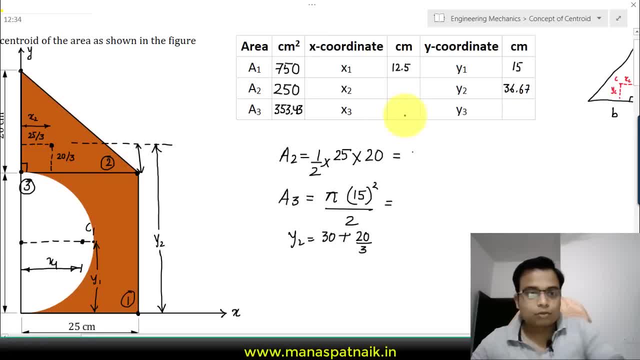 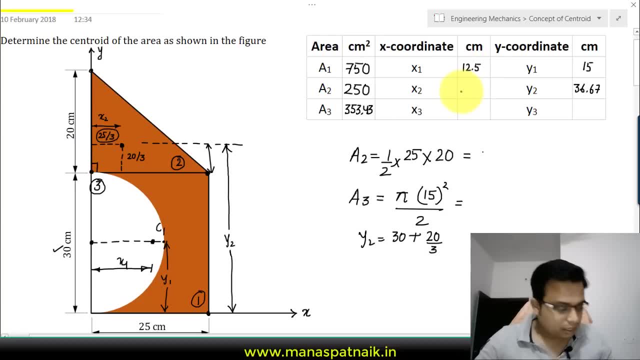 6.67.. Okay, so what was the value of x2?? Okay, x2 values was this: 25 over 3.. 25 over 3,. if you try to work this out with the help of a calculator, it's going to be 8.33.. 8.33.. Done, Okay, now let's. 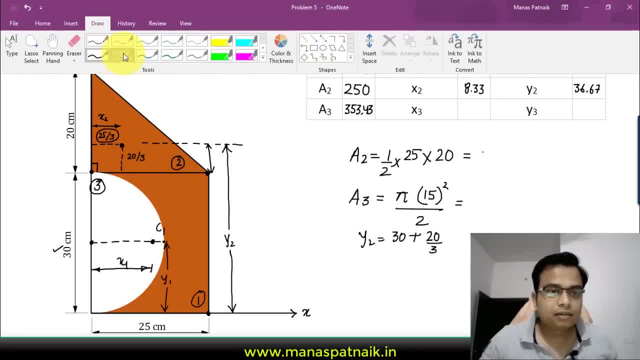 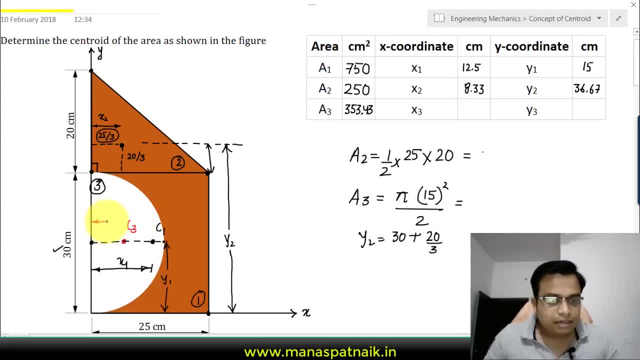 worry about this semicircle. Now, for that I'll be using a red color. Now, the semicircles centroid will be somewhere here, Okay, And this will be at a distance of, okay, it will be in the line of symmetry. this dotted line that I've made is the line of symmetry And in that line of symmetry, 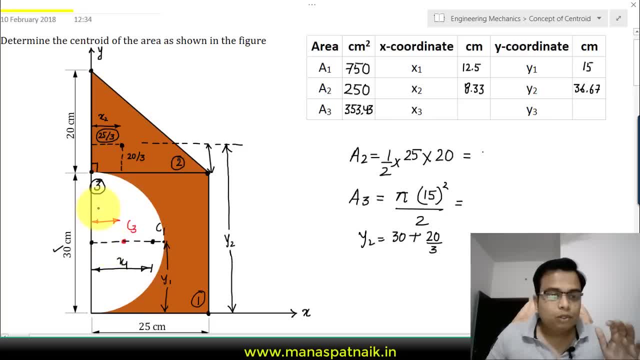 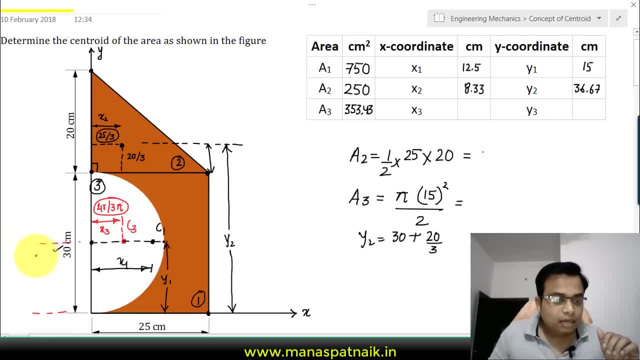 calculate the value of y3, it would be like this: this is going to be y3.. Okay now, y3 is pretty simple. This is: y3 is going to be equal to 15.. But what about x3? x3 is going to be equal to four. 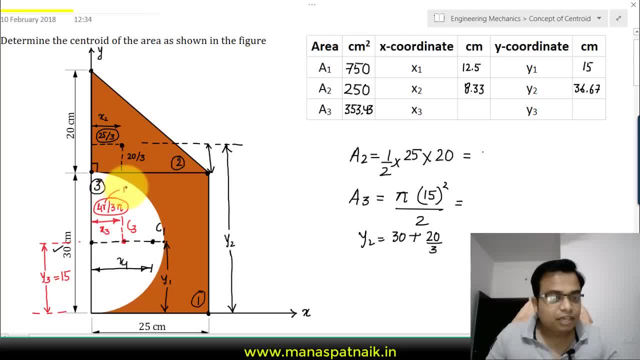 r upon three pi. So put the value of r, value of r is nothing but 15, right, put it over here. And the final value of x3 obtained will be equal to 6.37.. 6.37. And the value of y3 obtained is 15.. 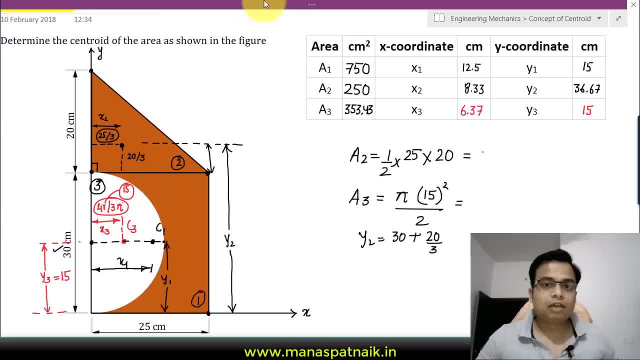 15.. That's it. Now, where is the rubber? I need a rubber desperately, man, And let me, let me- erase all of this stuff. Okay, Let us get back to the pen mode. Now what? what we need to do is: there is a rectangle and there is a. 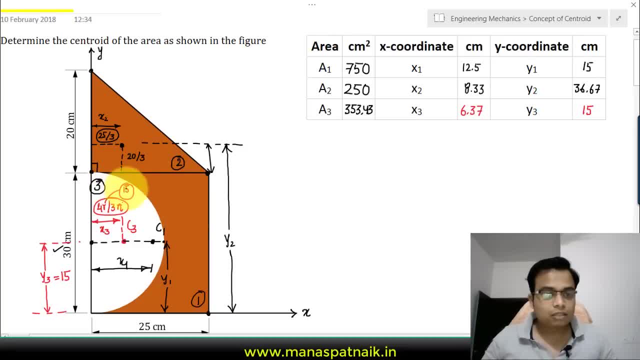 triangle, Okay, in combination, out of which a semicircle has to be subtracted. So, essentially, what I mean to say is one plus two minus three. Okay, so this is the approach that we're going to be following, And xc can be written as a one x one plus, a two x two minus. 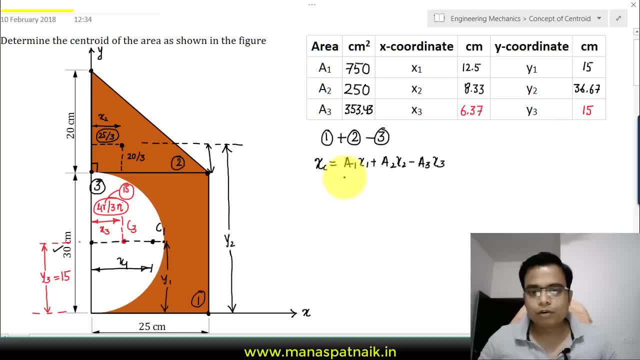 a three x three over, and that's A one plus a two, one plus two minus three, That is a three. In the same manner you can find this centroid: a centroidal y is equal to a one y one plus a two y two minus a three y three whole divided. 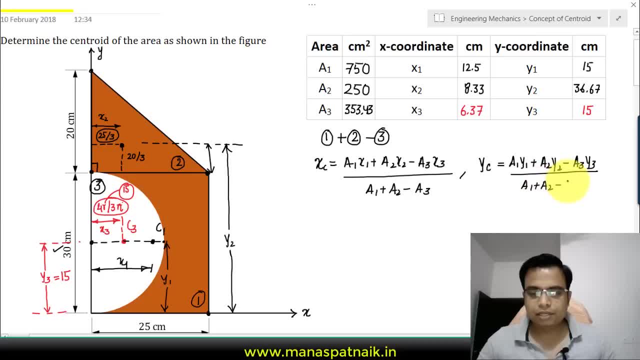 by a one plus a two minus a 3.. Now, guys, you need to put all these values- a 1, a, 2, a, 3 x, 1 x, 2 x, 3 y, 1 y, 2 y, 3- over here. here and the final: 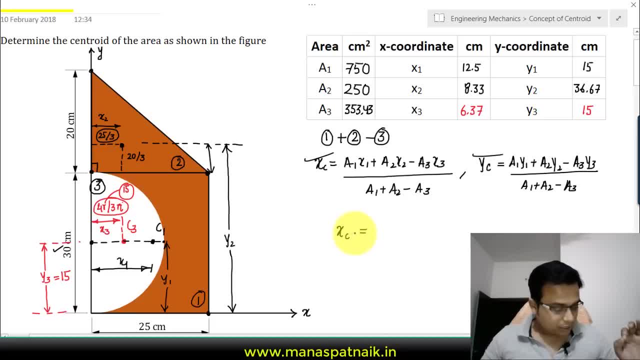 value of x, c is going to work out as 14.24, 14.24 centimeters, and the final value of y, c, centroid y, works out as 23.38 in centimeters, 23.38 centimeters. so, guys, that was all from my. 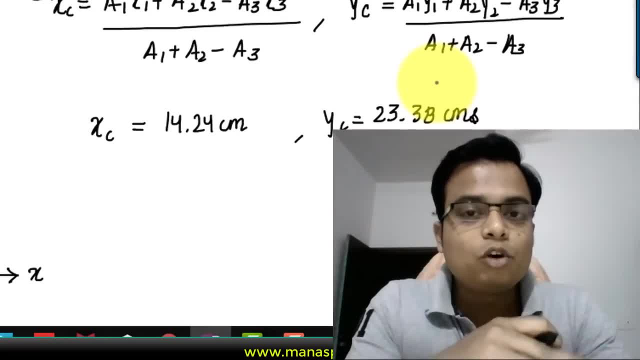 set for today. well, if you've got any doubt or query, do write them down in the comment section below. i'll be happy to answer them, and if you believe that this video tutorial has added value to your knowledge of mechanics, then do share and like this video, subscribe to this channel and.